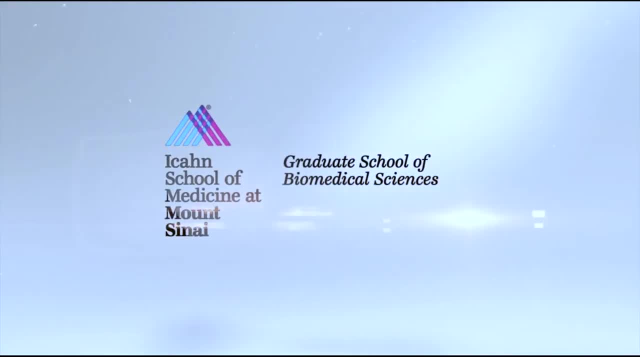 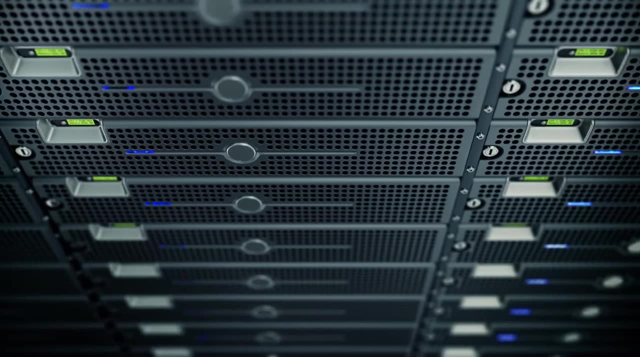 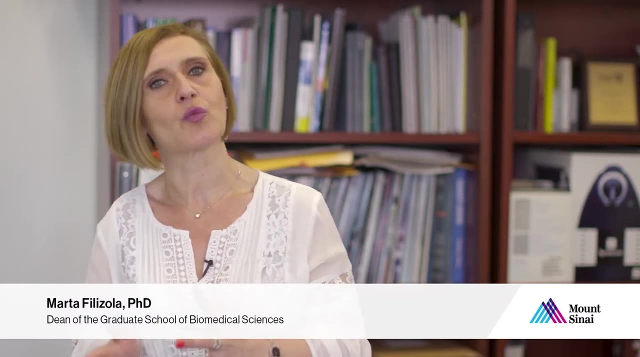 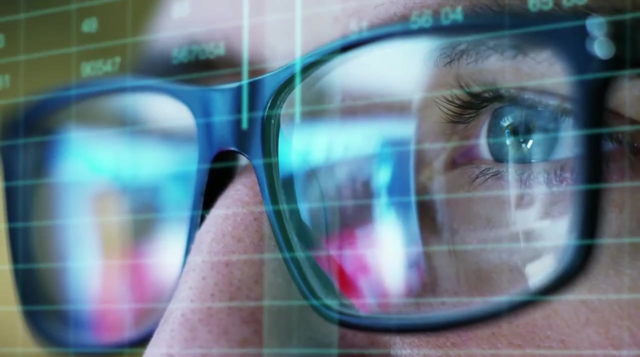 The Master of Science in Biomedical Data Science is a new master program, a new graduate program in the graduate school that will be combining a training in biomedical sciences with machine learning and big data analytics. The idea is to expose students with a strong quantitative background to complex biomedical programs. We're looking for students who have major. 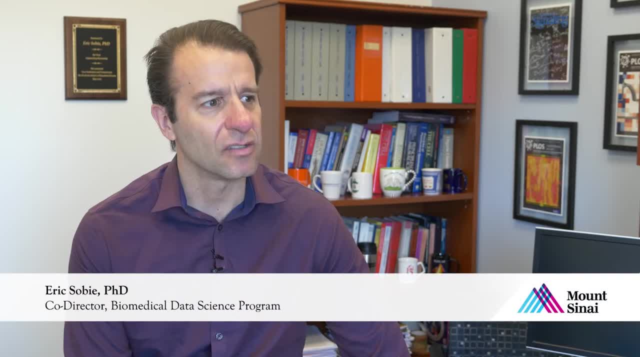 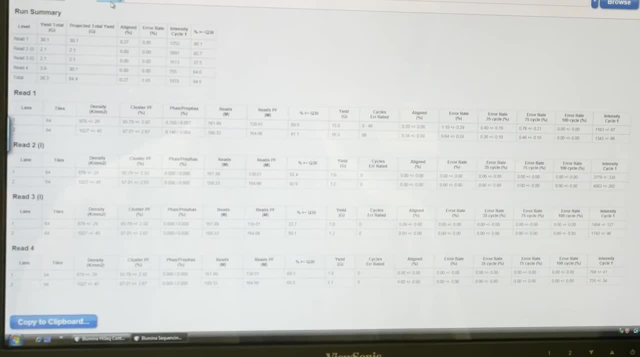 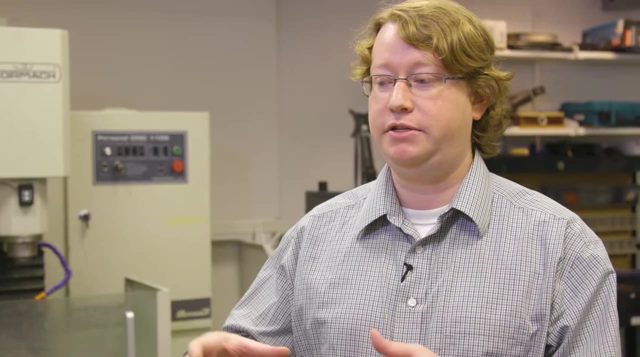 and undergraduate disciplines such as computer science, engineering, physics, those kinds of disciplines, but those who have a real desire and passion to want to work in the healthcare realm. What we do typically is students will do research within a lab that provides sort of the core foundation and the domain topic area of their 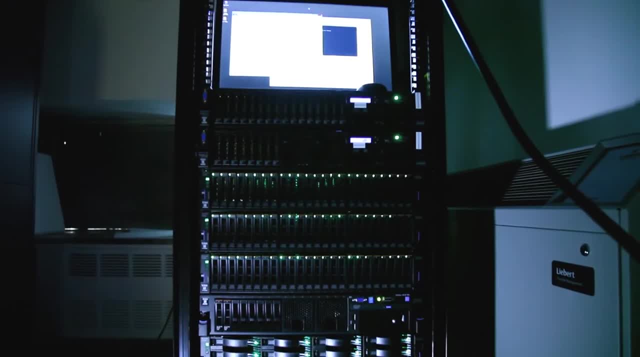 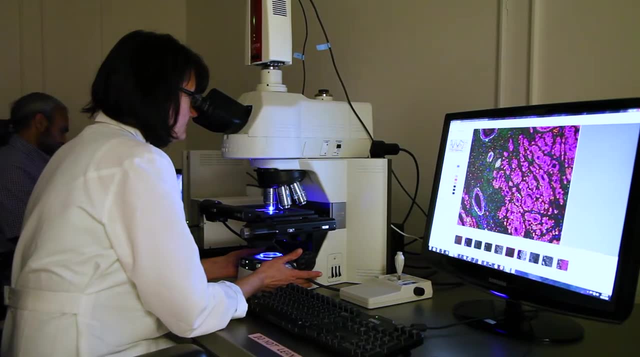 interest and then that's integrated with coursework in things like computer systems, in things like machine learning algorithms, biomedical data science, of course, statistics and engineering, In order to give them the sort of computer and data science foundation necessary to go out to these programs and make use of their data. 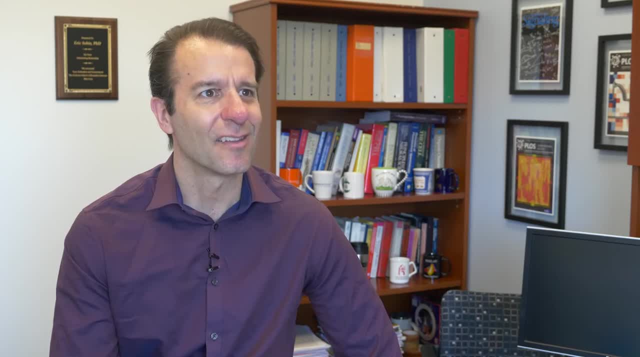 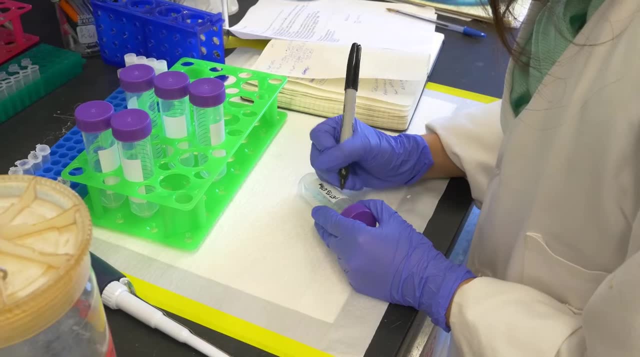 Students who graduate from our program, the Masters of Science in Biomedical Data Sciences, are going to be poised to address difficult problems, specifically in the healthcare and biomedical science communities. One of a number of different types of labs that would be appropriate for work for a master. 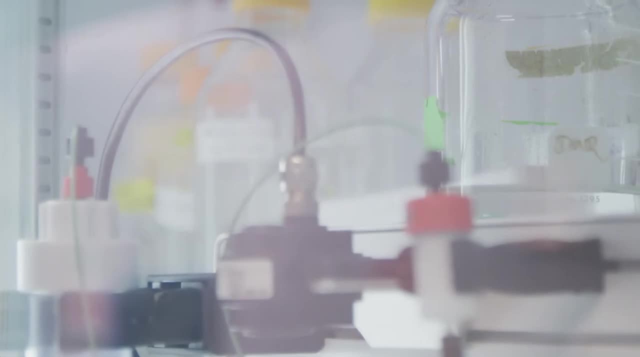 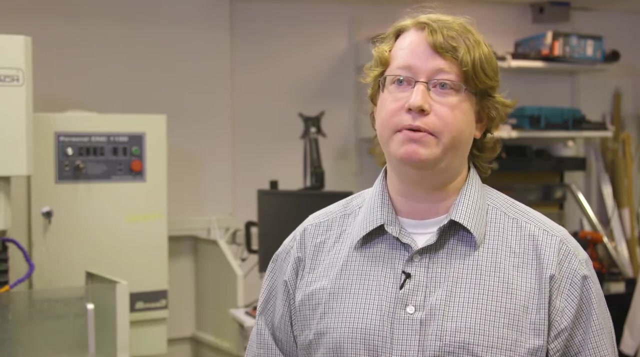 student who comes into the group. we're a biomedical engineering group, but there are many other types of institutes and other kinds of research possibilities within the school. We're expanding the entire gamut of all possible health data that's generated here at Mount Sinai. 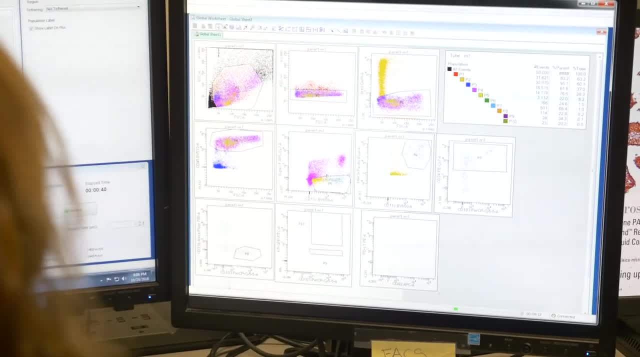 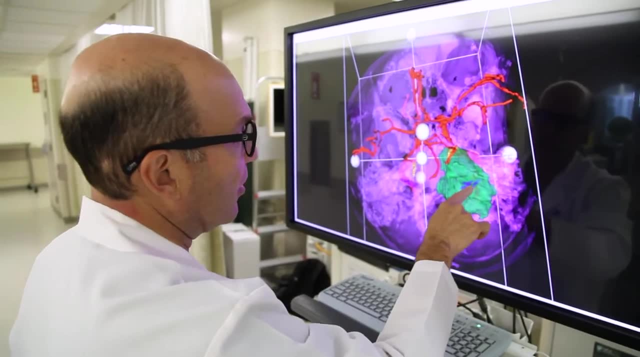 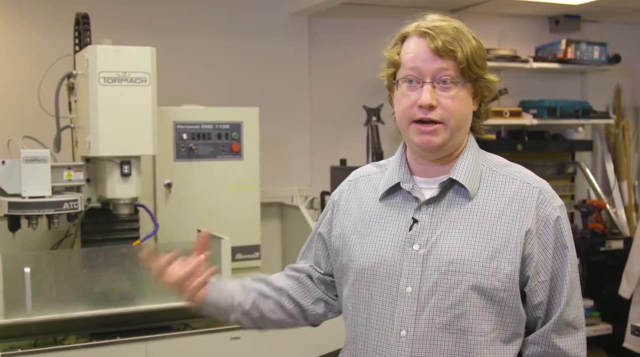 This coursework will be combined by a capstone project that will be mostly focused on a complex problem that is currently being tackled by one of our several faculty. We take advantage of the kinds of programs and our relationship to the entire health system here at Mount Sinai. 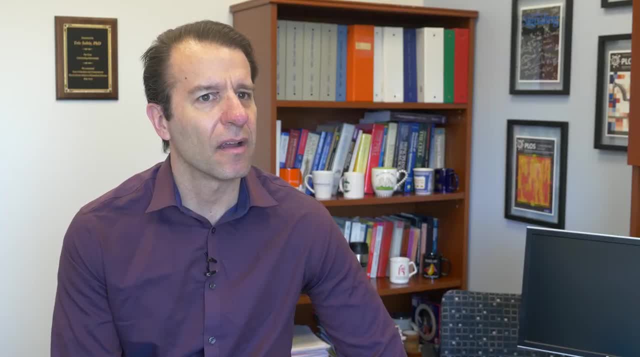 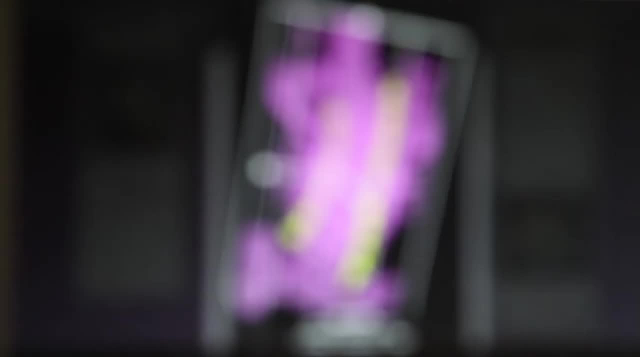 Mount Sinai is a unique environment because we are a graduate school that is embedded within a hospital. One of the reasons that I like programs like our master's program here is that it brings people who now have the opportunity to build the kinds of expertise in the area and then